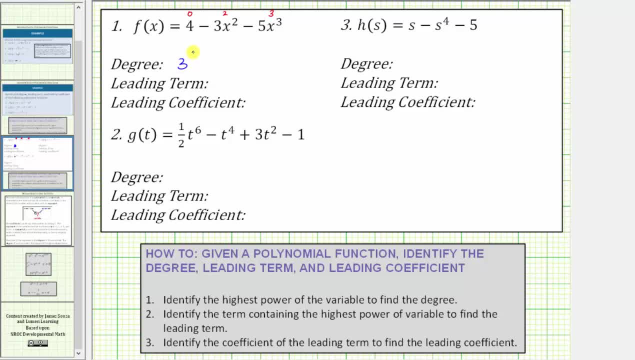 polynomial function And because the term containing the highest power on the variable is negative five x cubed- negative five x cubed is the leading term. The coefficient of the leading term is negative five and therefore the leading coefficient is negative five. Now I do want to mention one more thing. 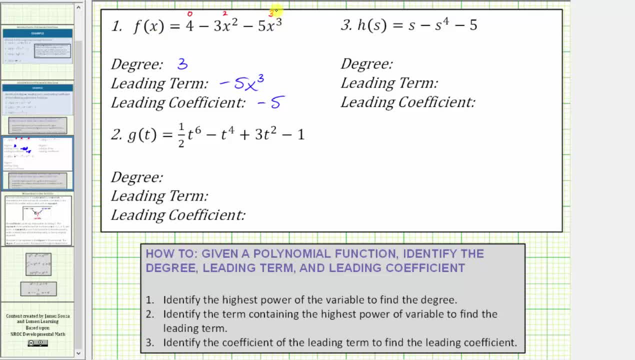 Often a polynomial is given in descending order, which means the terms are listed from highest degree to lowest degree. If you were to write f of x in descending order, we would have: f of x equals negative five x cubed minus three, x squared plus four. One nice thing about. 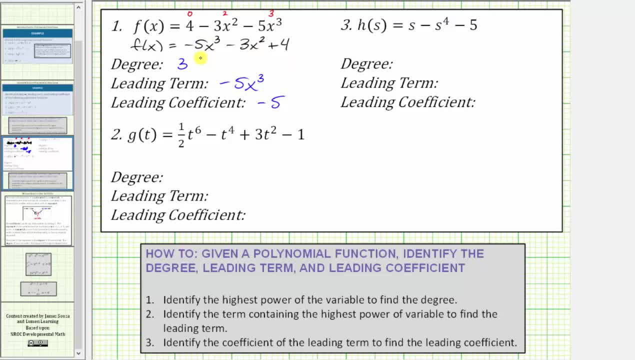 having a polynomial in descending order is that we can determine the degree, the leading term and the leading coefficient from the first term of the polynomial function. Again, as long as it's in descending order. Number two: we're given g of t equals one half t to the sixth minus t to the fourth plus three t squared minus one. 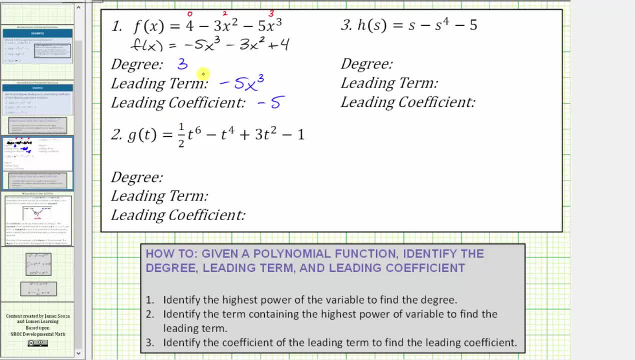 Let's begin by determining the degree of each term. The degree of the first term is six because of the exponent of six on the variable t. The degree of the second term is four, given by the exponent of four on the variable t. The degree of the third term is two. 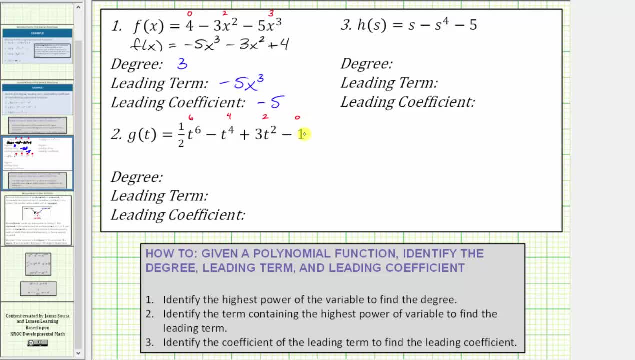 the degree of the last term is zero. Because the highest power on the variable is six- this is a degree six polynomial function- And because the term containing the highest power on the variable is one half t to the sixth, the term one half t to the sixth is: 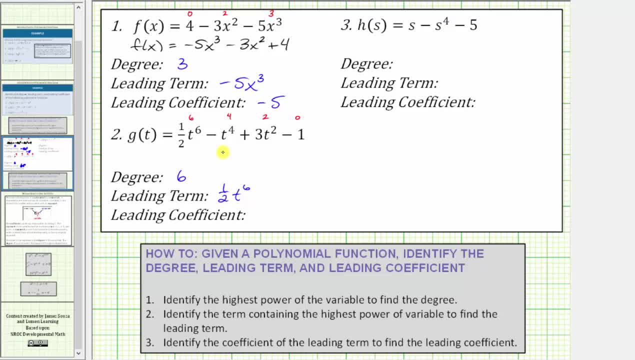 the leading term And because the coefficient of the leading term is one half, the leading coefficient is one half. Notice, this time g of t was given to us. in descending order Number three, we have: h of s equals s, or if we 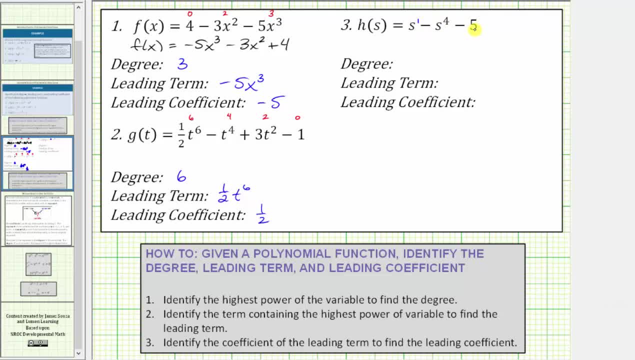 want s to the first minus s to the fourth minus five. The degree of the first term is one given by the exponent of one on the variable s. The degree of the second term is four, given by the exponent of four on the s And the degree of the constant term negative five.